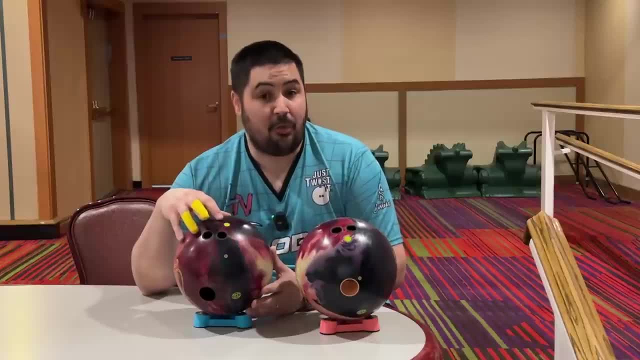 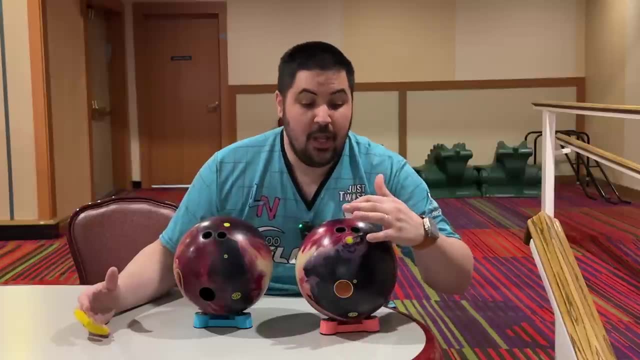 them is pin up. one of them is pin down. The pin up one is 30 by four and a half by 30.. The pin down one is 30 by four and a half by 70. That 70 is what made it go from pin up to pin down. So let's. 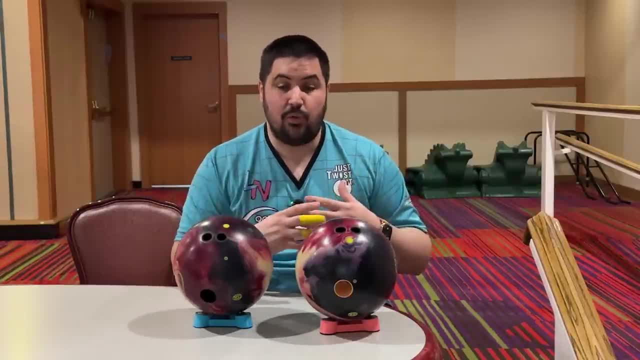 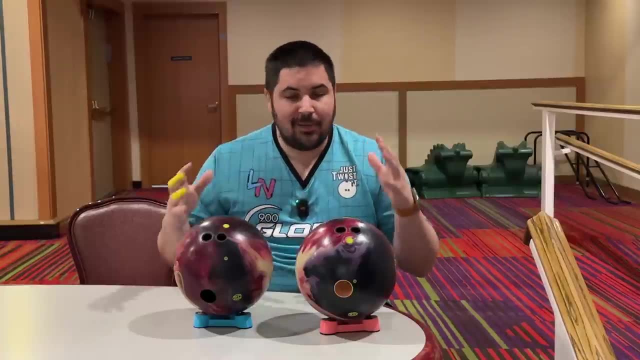 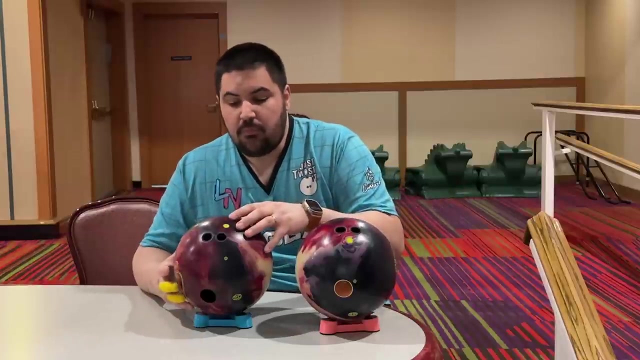 talk about the science behind what happens to the core numbers of a bowling ball when you drill them up versus when you drill them pin down. And we're going to do, in layman's terms, very simple, because there's no need to overcomplicate a ultimately simple idea: When you draw a bowling ball, pin up. 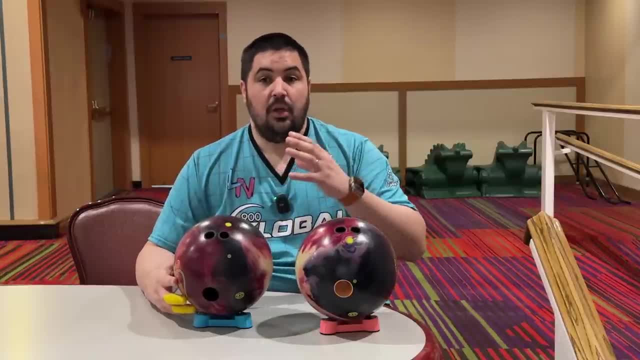 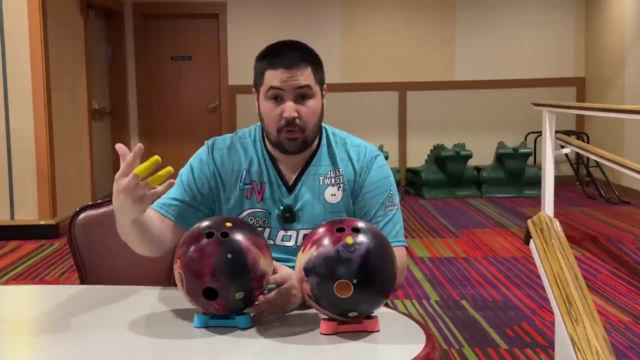 okay, the differential. which? the differential means? it's hooked potential. So the differential is going to go up. Okay, so the hook potential is going to increase And it's RG. the RG stands for radius of gyration. the RG is going to go down. 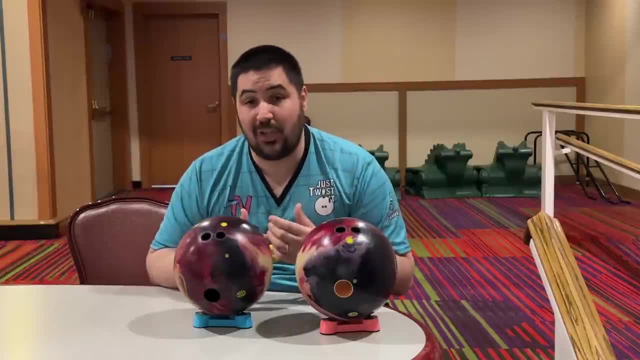 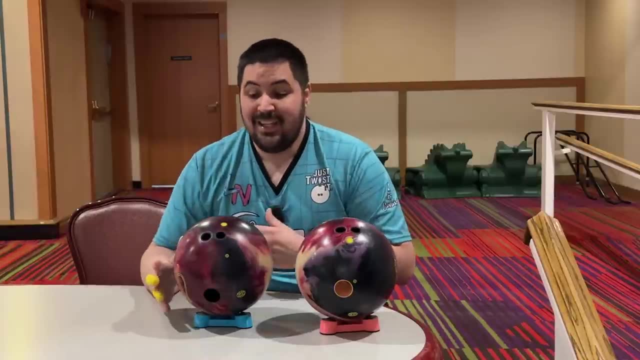 The lower the RG, the earlier the ball is going to want to pick up. the higher the RG, the, you know, the longer, in layman's terms, the longer the bowling ball is going to want to go. And so, because it is, 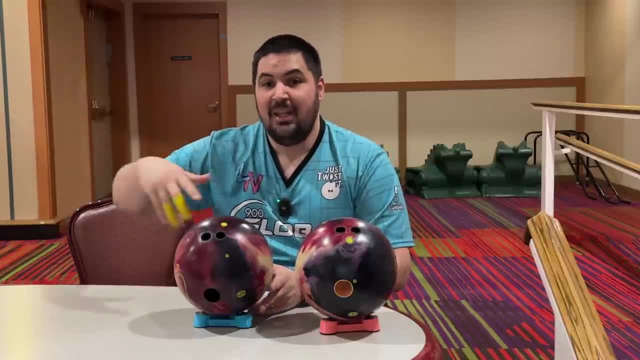 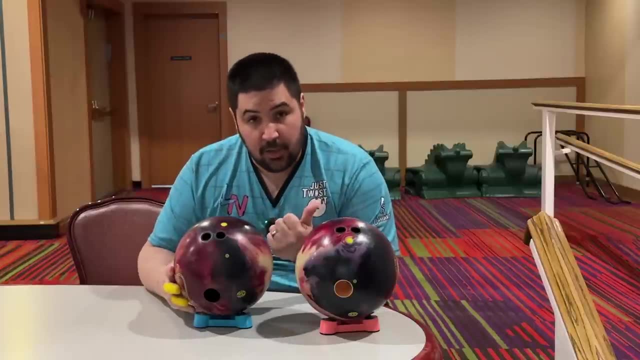 a lower VAL angle, which is that last number, the 30,. it's going to want to change directions pretty quickly. So the ball in general is going to be earlier, it's going to be stronger and it's going to shape a little bit more down lane. 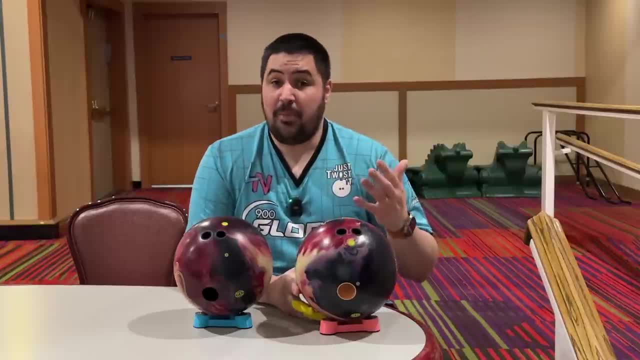 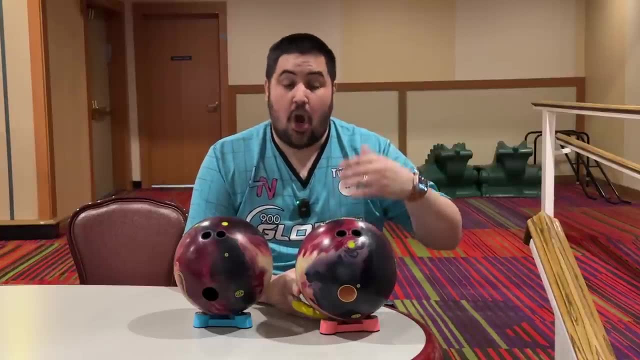 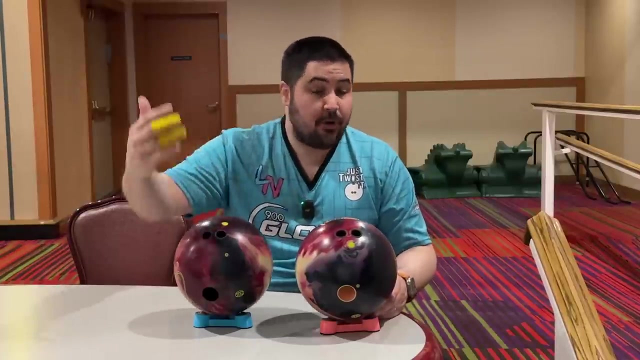 Then, when we turn it over to the pin down, it's going to be just the opposite. the differential, or its maximum hook potential, is going to decrease, its RG is going to increase. So it's going to want to be a little bit, it's going to hook a little bit less, it's going to go a little bit further. 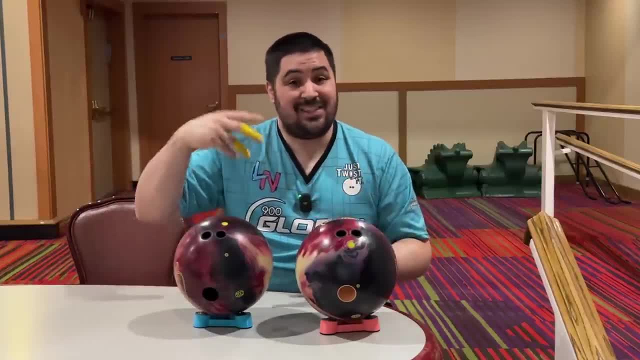 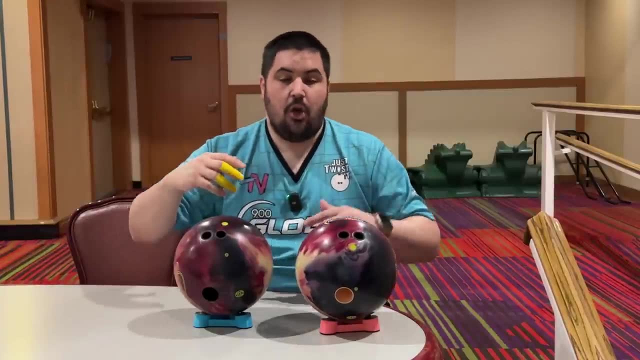 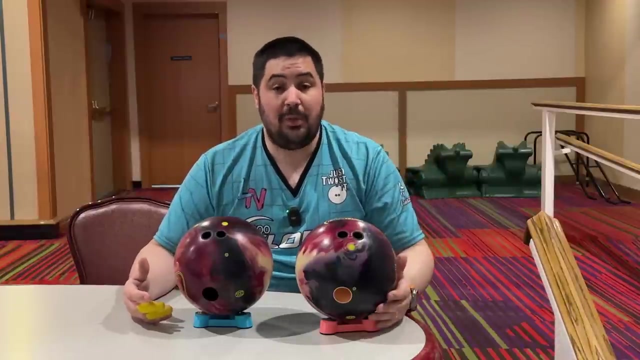 down lane And then that VAL angle be being 70, it's going to increase that number. the higher that number, the rounder that ball is going to want to be. So in general, the pin down bowling ball is going to be longer, it's going to hook less and it's going to be 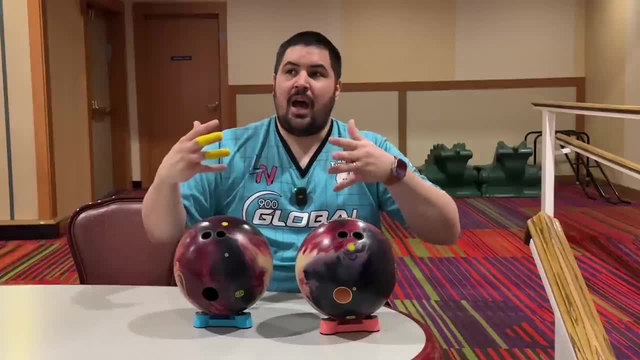 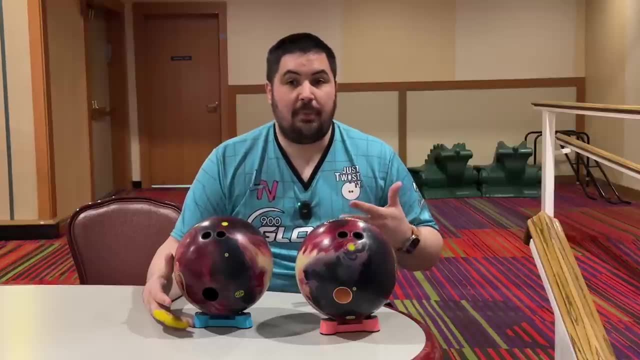 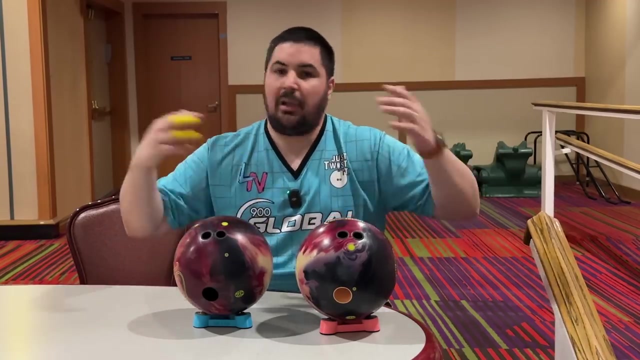 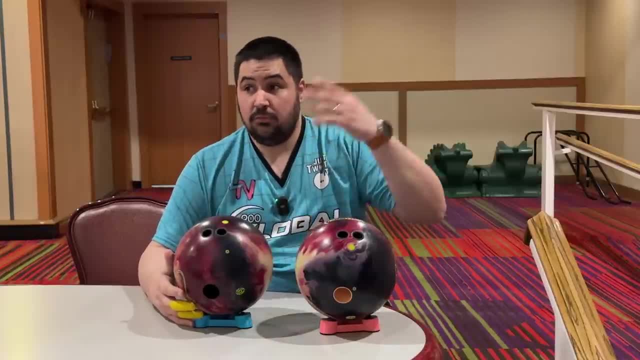 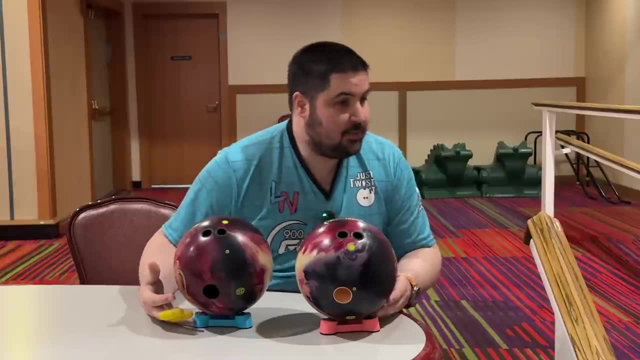 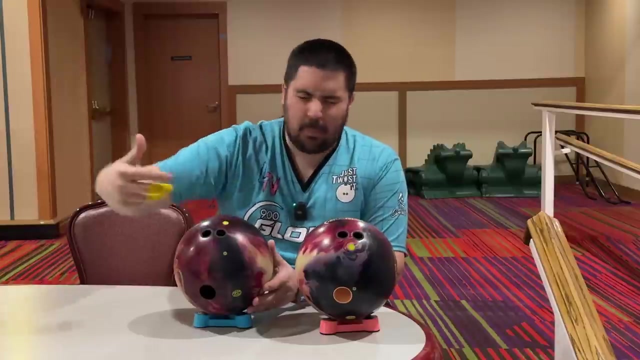 like this: The core does not touch the lane, Obviously the cover does. So the surface of the bowling ball is going to be the biggest, biggest, biggest deciding factor. You can take a layout that's meant to go super long, super quick down lane and hit it with a 500 pad. 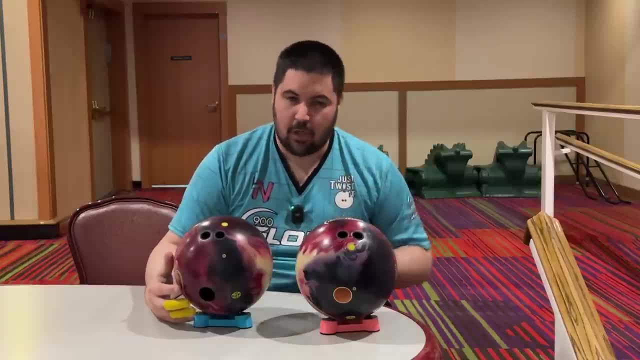 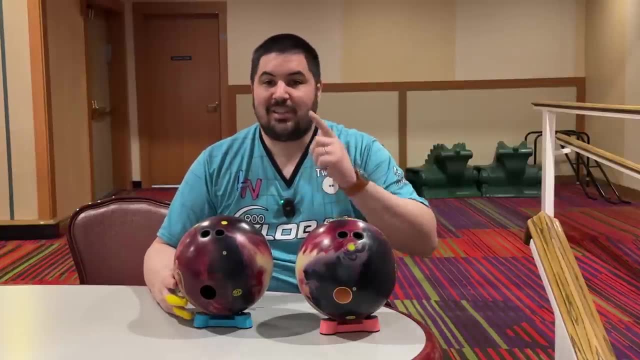 and it's going to be earlier and smoother than a ball that's drilled to be early and smooth that doesn't have a whole lot of service on it. So be very careful when always asking about layout when sometimes you should be asking surface- And I know this is a super 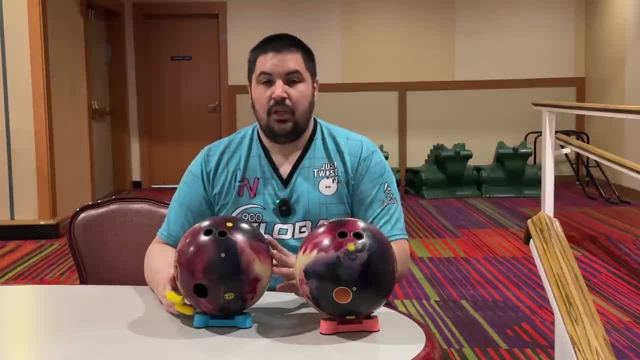 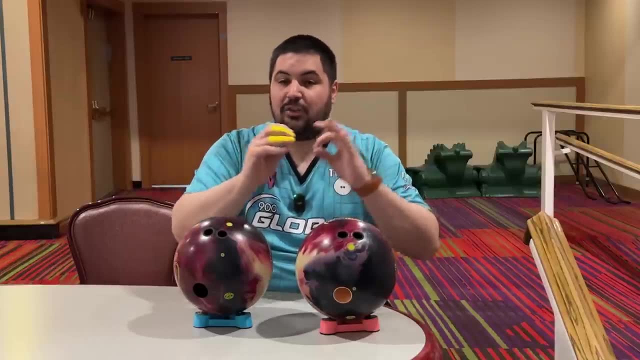 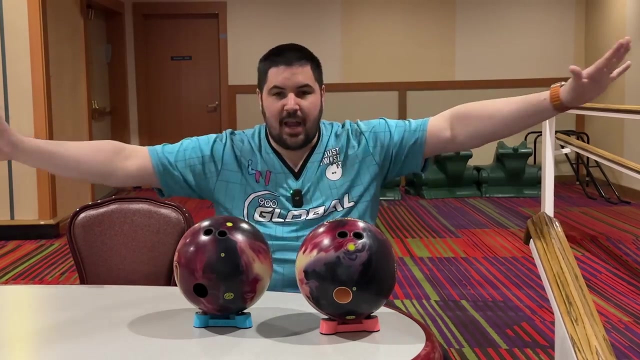 long introduction, But I really need you guys to understand that Surface is going to end up being the largest deciding factor when it comes to ball motion. The layout is just going to fine tune that, so you have to use both of them in unison. So all of that out of the way. 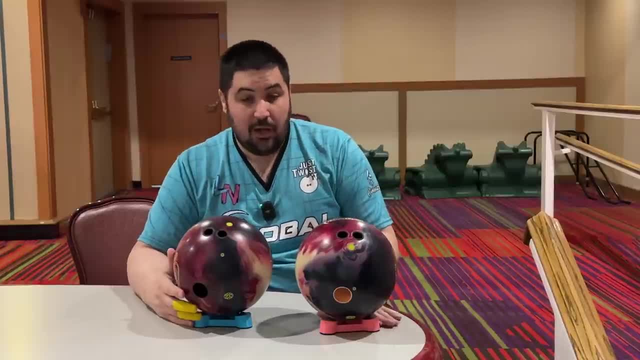 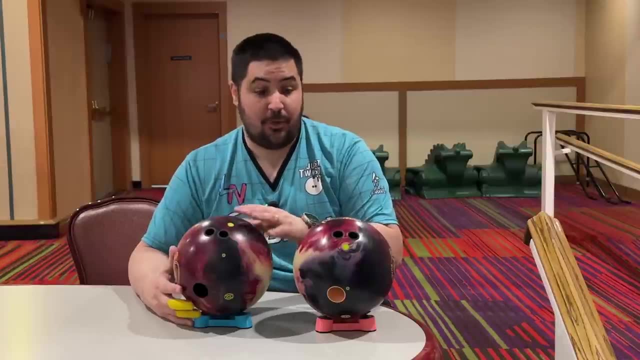 When can you use each of these bowling balls? Well, it's bowling. you can use them at any time you want right? I've had success throwing pin up bowling balls like this on the fresh. I've had success throwing these pin down ones on the fresh, and vice versa. 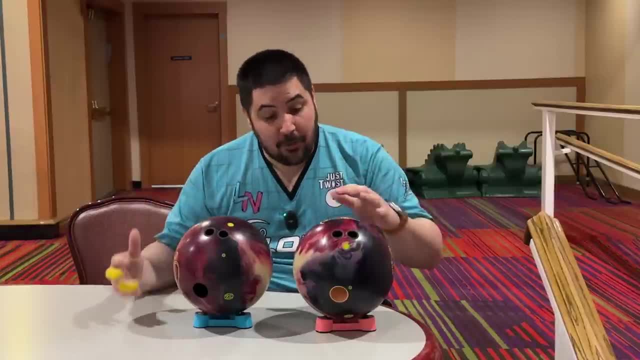 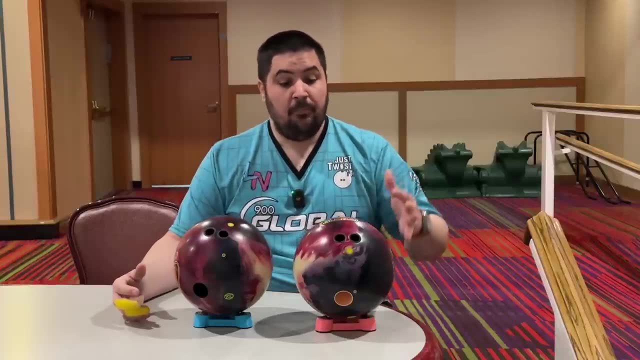 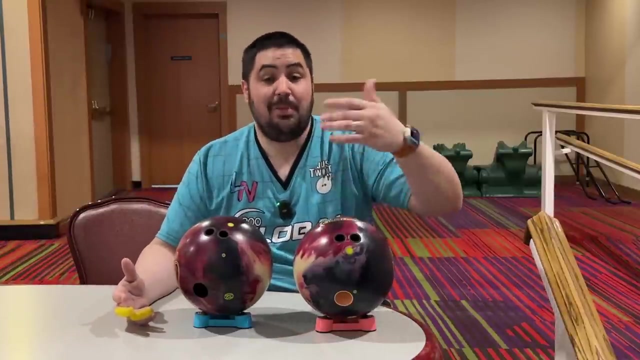 But for me in my game I would prefer to throw the pin down ball on the fresh. Why It's longer, it hooks less and it's smoother. On house shots there's already a ton of friction to the right, like there is here at Samstown, So because of that I like a bowling ball that's going to hook. 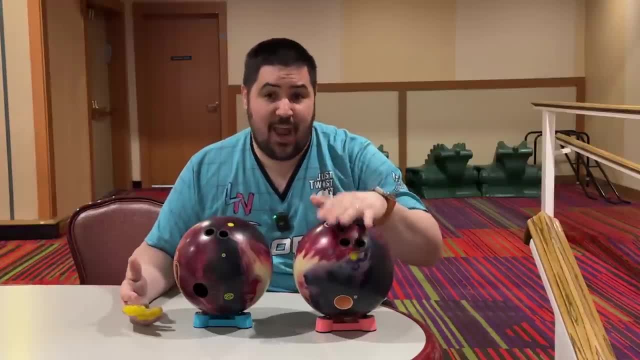 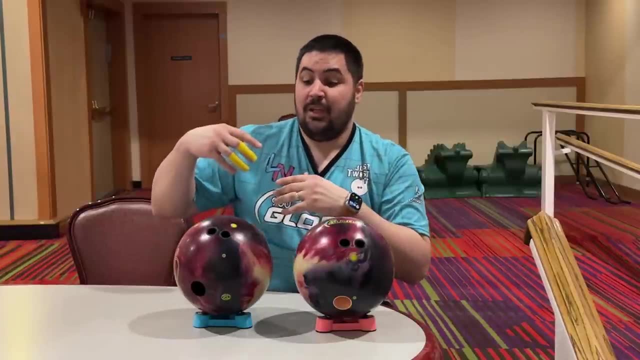 a little bit less, a little bit smoother down lane And that's why, for me, I, if I have one in the bag, I prefer the pin down one on the fresh, then the pin down one or the pin up one, rather, Even though that RG is going to go down and that differential is going to go up and it's going to. 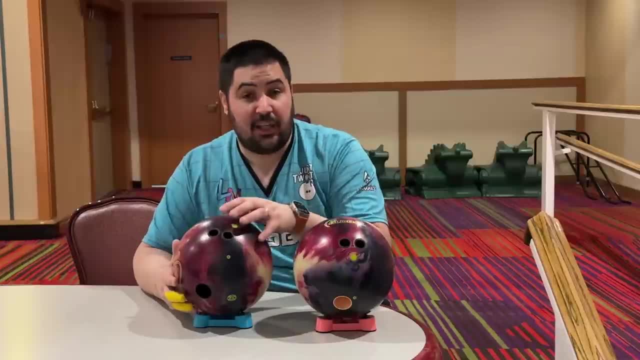 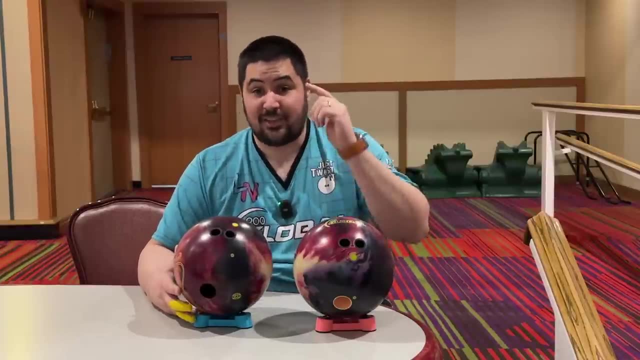 want to be quicker down lane. I have typically liked throwing these kind of layouts with these kind of bigger bowling balls In game, three in league. if you guys have been watching my league live streams, which is every Tuesday night at 7pm Pacific Standard Time, I've been throwing a magic. 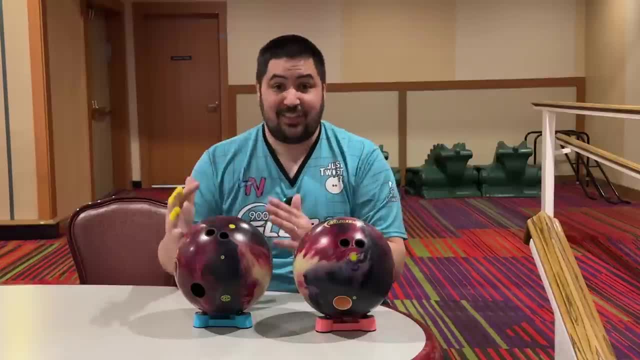 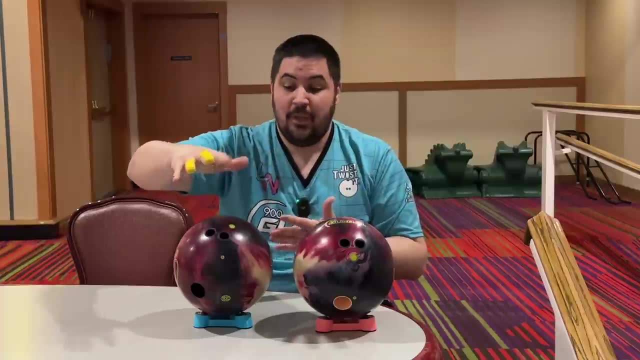 bag with a lot of surface, game three in League because it hooks instantly And then it kind of just bails down lane because of all the friction As you develop all this carry down where the bowling balls are going down the lane. you kind of want something that's going to be a little 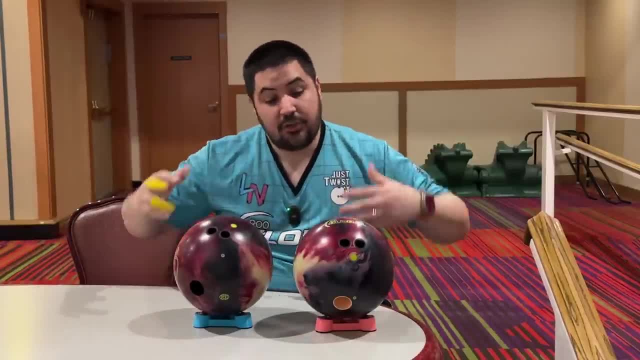 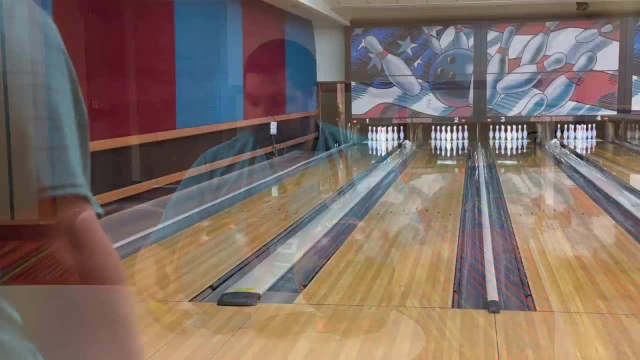 bit earlier and it's going to hook before all that carry down. So for me, pin down on the fresh, pin up in transition in general. We'll see you here on the lanes. Alright, we're going to start in the pin down one Again: longer, smoother, less hook overall when compared to that pin down ball one. 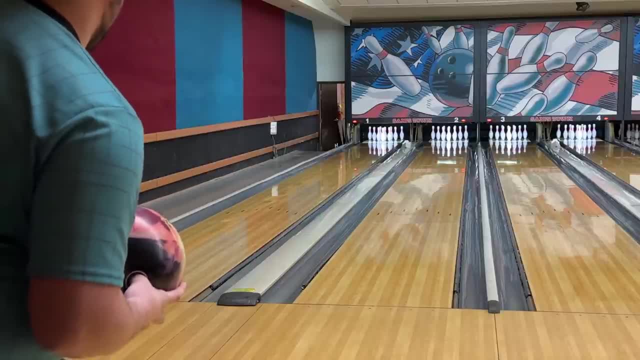 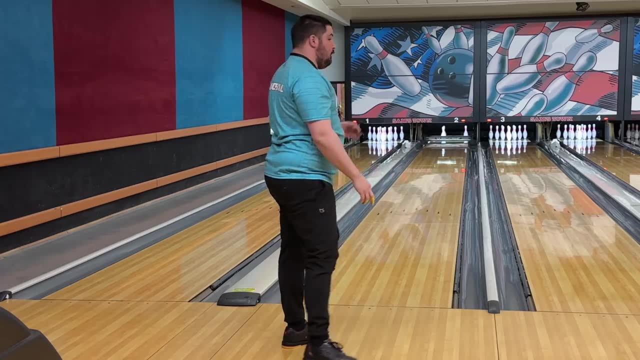 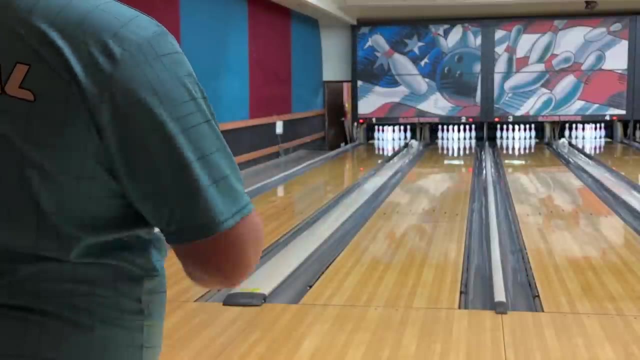 up one. so let's start this one, establish a baseline. so that was literally the first shot on this lane. i'm gonna have to move right off that for sure. so i'm gonna move like four right off that shot because it was not even close but, like i said, it was literally the first shot on. 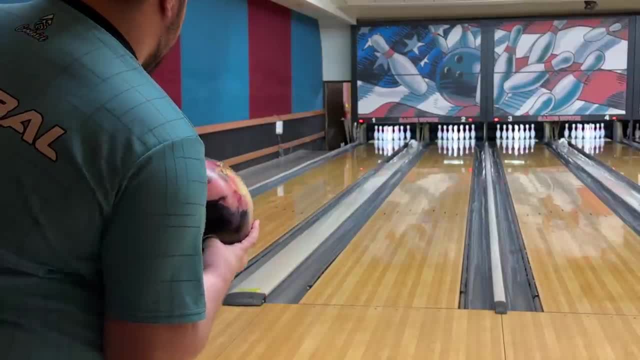 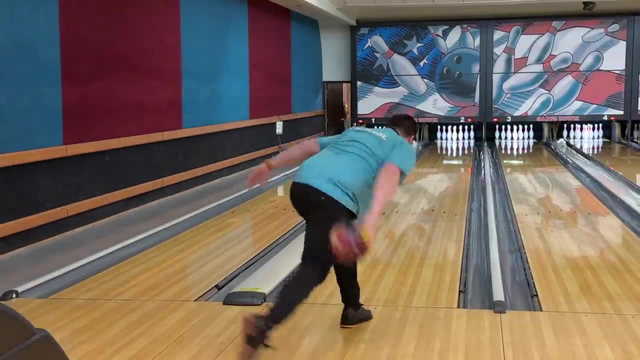 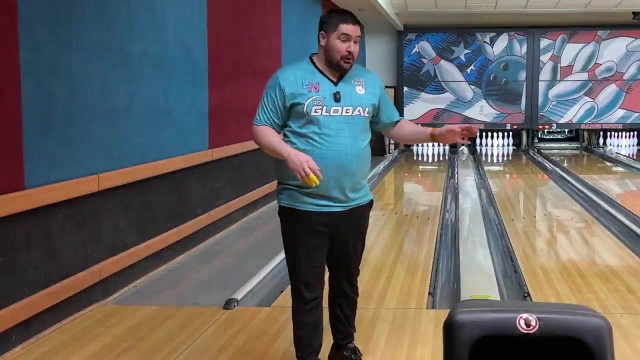 this lane, so move everything like four and two right, nice and straight up the lane here. see this freaking lane man. all right, so you guys saw what happened there on lane two. needless to say, i'm not going to throw any more shots on lane two. i've had issues on that lane. 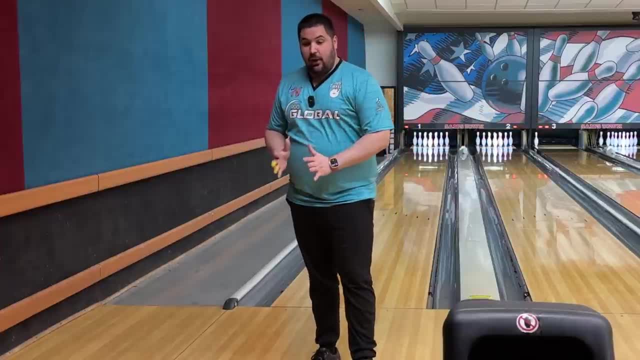 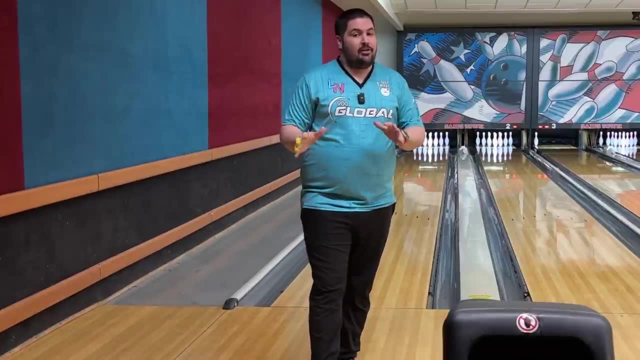 last couple months. so we're going to sell lane one, which we know is super nice. so we're going to go to the spot where i 2, 8, 10 on lane two. lane one is a little bit more transitioned because i did film a video before this, so they're going to be a little bit more transition. 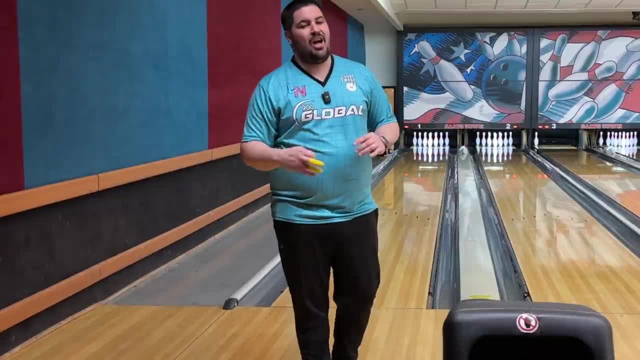 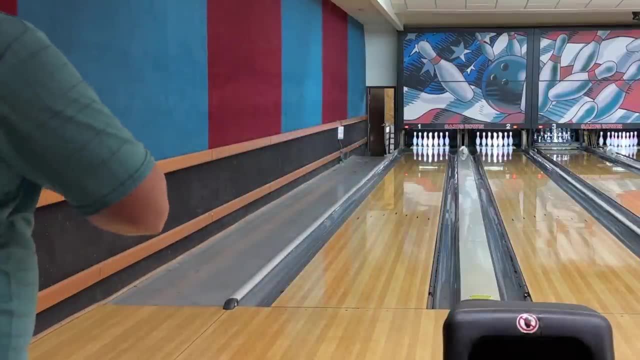 but it should be fine. not, i'm bowling by myself, not. a whole lot of shots went down the lane, so we're going to turn it around now and get on lane one, all right. so here's the not sticking and almost dying. so we're going to go to the spot that we 2, 8, 10 on lane two, just to see. 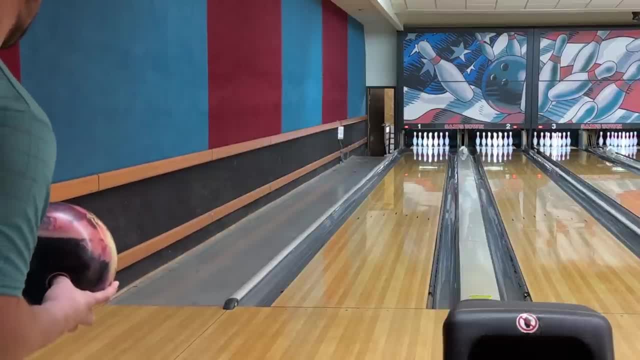 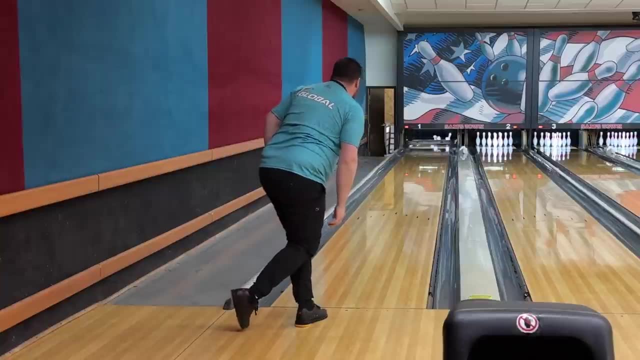 it should hook here, since there's more shots thrown on lane one. yeah, so lane one hooks way more. that looked pretty good. it was a little slow, but it was a little bit slow, so we're going to go to the spot where we 2, 8, 10 on lane two. 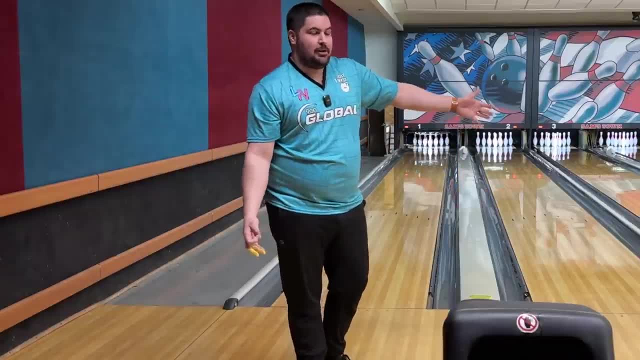 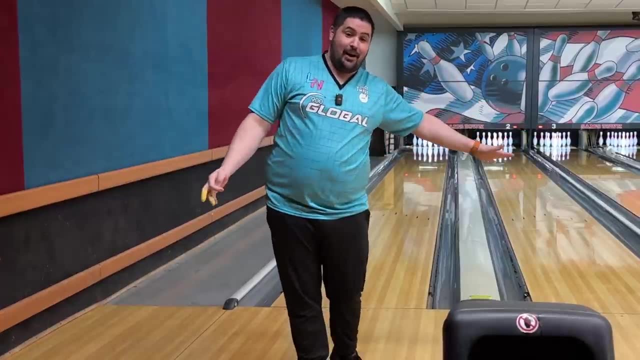 slow, a little hesitant, because obviously what just happened? i thought i was gonna, i literally thought i was gonna die. i was talking to my my friend tim here. how many times can i do that before i fall? and i hope it's uh never get stuck again like that. so we're gonna move. stay in the. 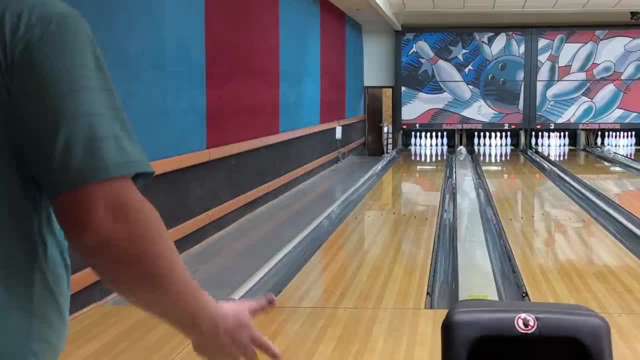 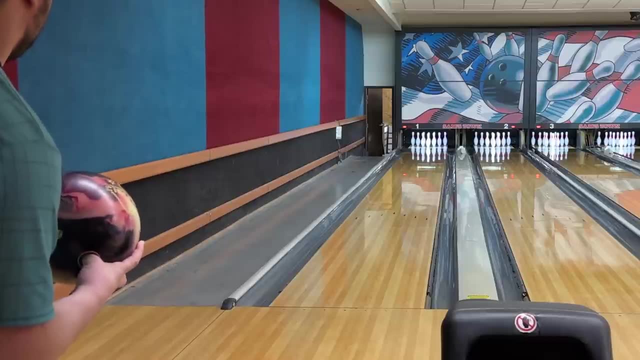 same spot, just get a little bit more aggressive after it. all right. so same spot, same spot, just a little bit more. a little more aggressive, a little bit more firmer, now that we know we're not going to stick and we'll go to the pin up line. 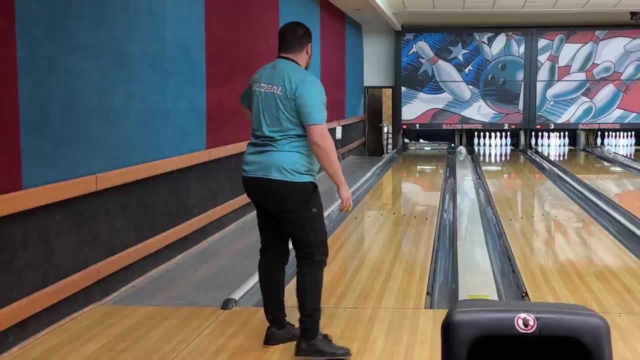 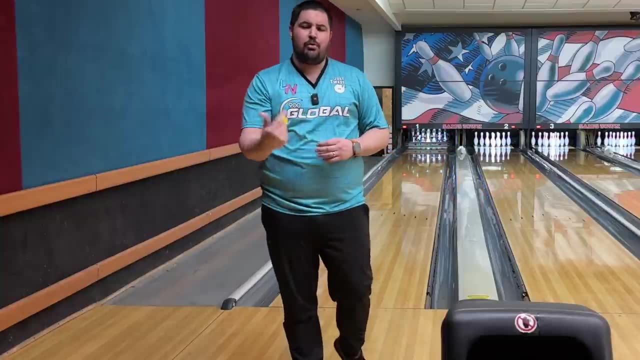 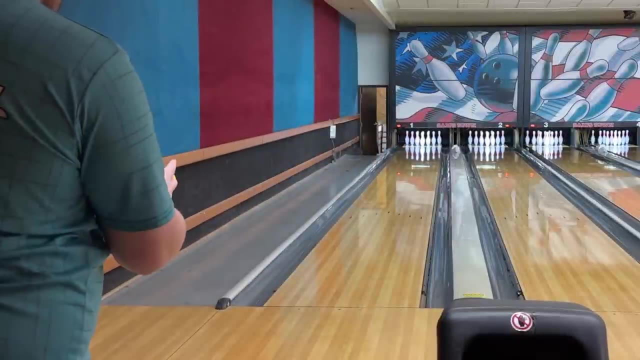 you can see the ball still hooks a lot. it's still an eternity pie, but it's a little bit cleaner than normal for asymmetric solids. very smooth down lane. now we go to the same spot, but in the pin up one all right. so i'm gonna do my best here to throw the exact same shot with the pin up eternity pie. 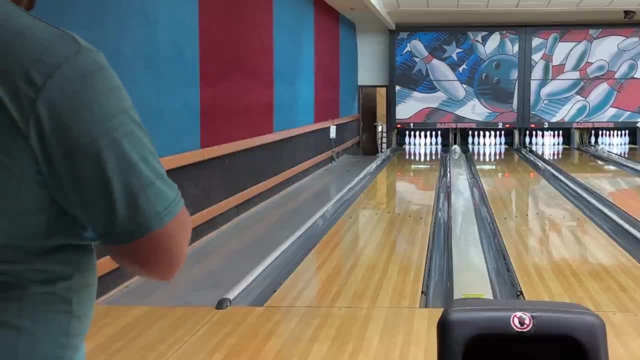 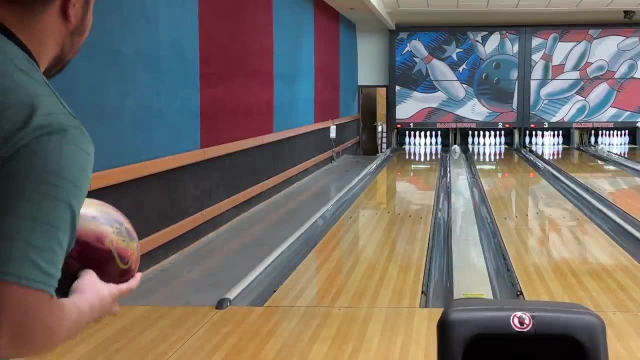 you're going to notice that the ball is going to want to get into a roll a little bit more, and it should. it should. if i throw it, the same should hook a little bit more. it might still strike, but it definitely should go a little bit higher in the pocket. 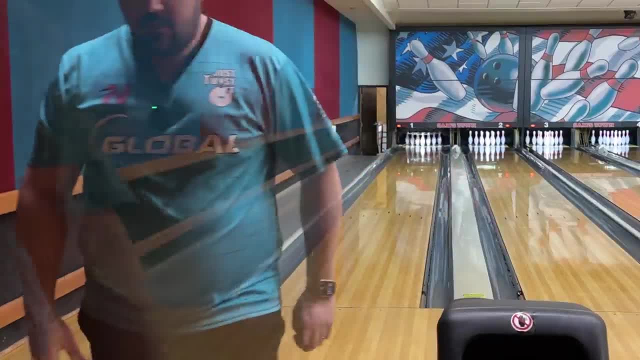 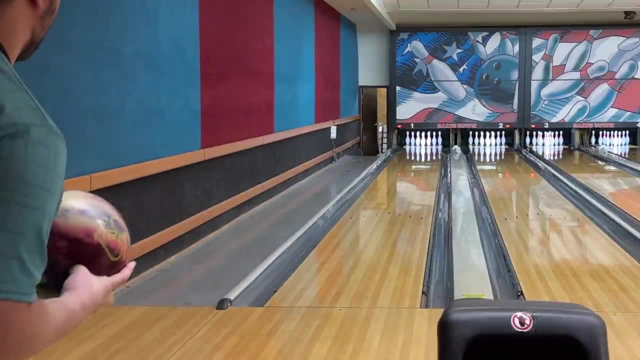 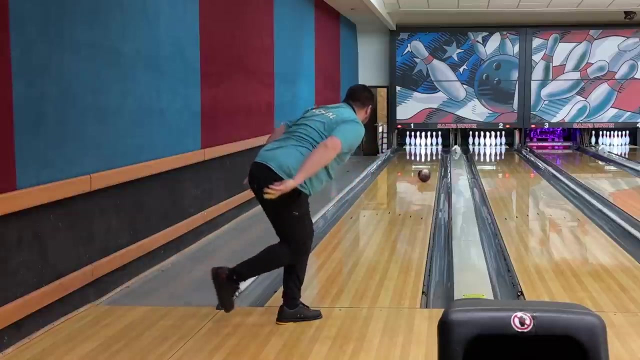 threw that bad, missed in wicked messenger. all right, so let's uh throw a better shot. that was, uh, not a not a very good pitch. the the flare lines on the ball are way different, so i'm going to throw a little bit more, and i'm going to throw a little bit more. 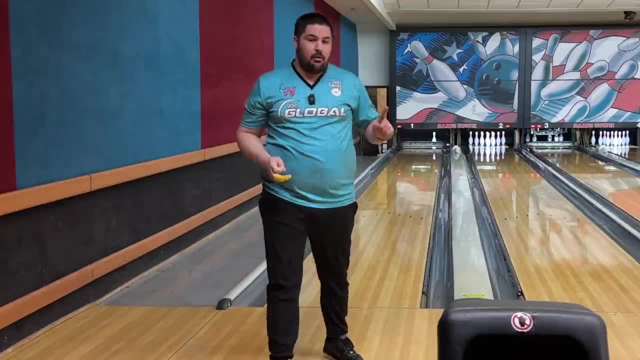 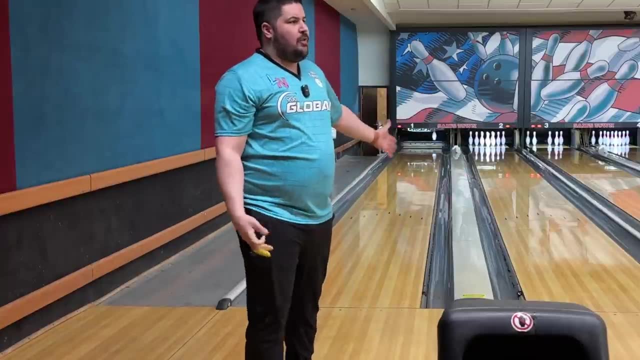 and i'm going to throw a little bit more, and i'm going to throw a little bit more. there we go, so that i threw that one much better, much closer to where that pin down was and you can see it hooked way earlier and way more so off that i'm going to move like maybe four left. 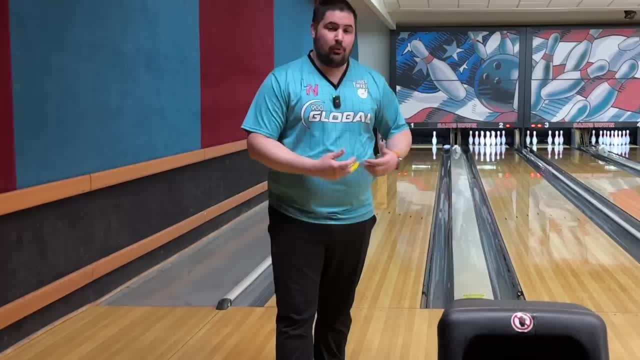 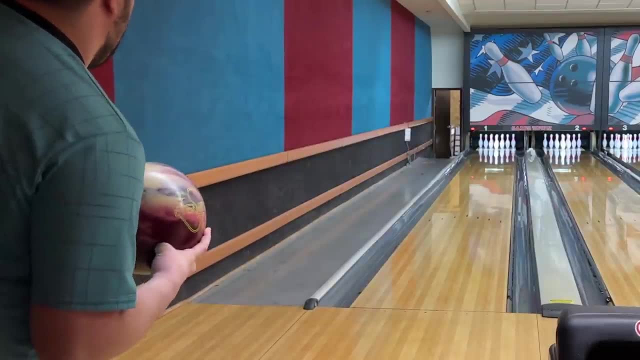 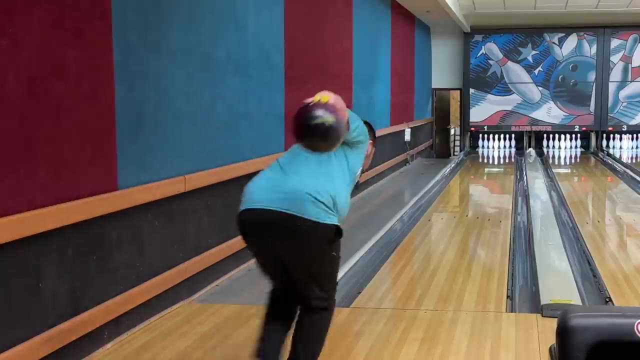 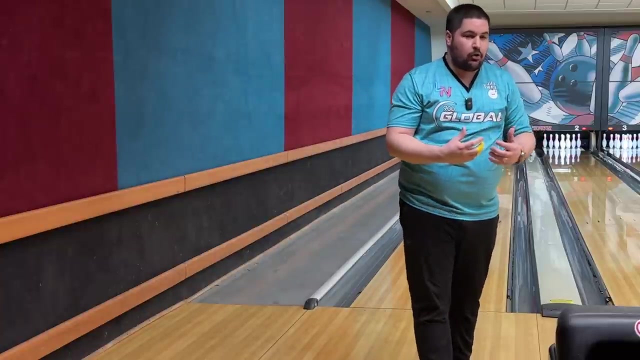 just really create a little bit more shape. let that higher differential really take effect here. so we're making that move like four and two ish really show you guys how the pin up one just hooks that much more. now the reaction is pretty good. yeah, way further left, creating much more traction in the oil. now we're going to get back to the pin. 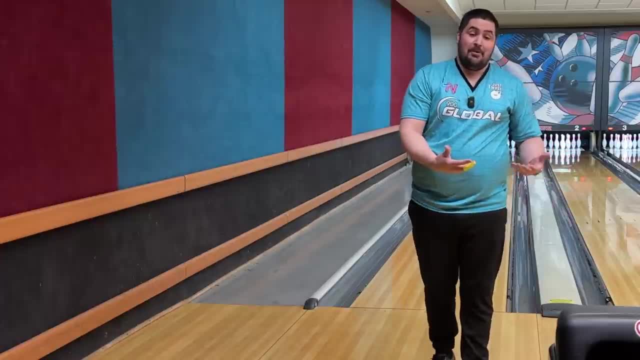 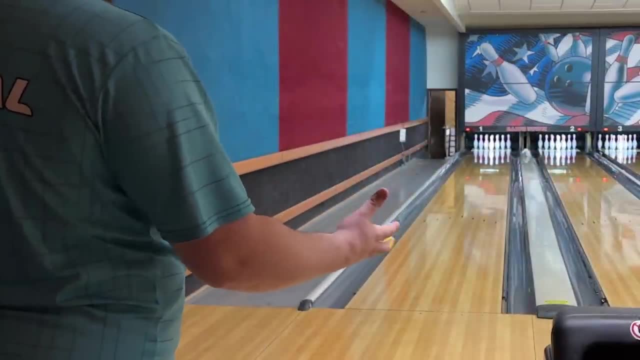 down one and just stay a little bit straighter, because it is going to allow me to play a little bit straighter and ultimately, that's what i want to be doing anyway- is playing straighter. all right, so now we're going to make that move back to the right with the pin down one and, like i told you guys, i prefer this on the fresh because it's going to allow me to play a little bit straighter. 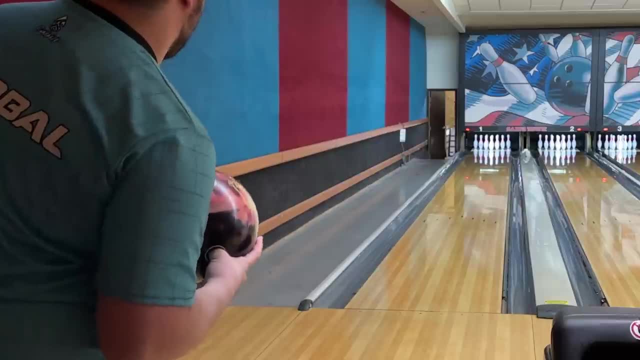 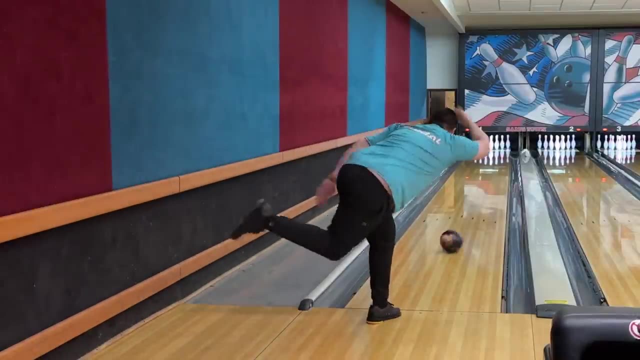 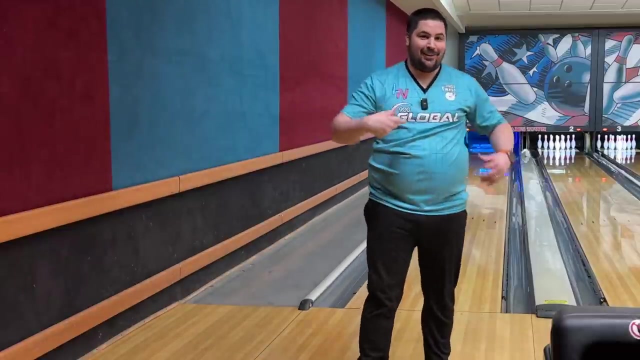 straighter, which is my a game. as you guys know, i'm trying to hit like 9, 10, 11 ish down lane like right, there is exactly the part of the lane that i'm wow. did you see where that exited the pin deck? that was pretty disgusting, but that's the motion i like on the fresh: clean, very smooth. 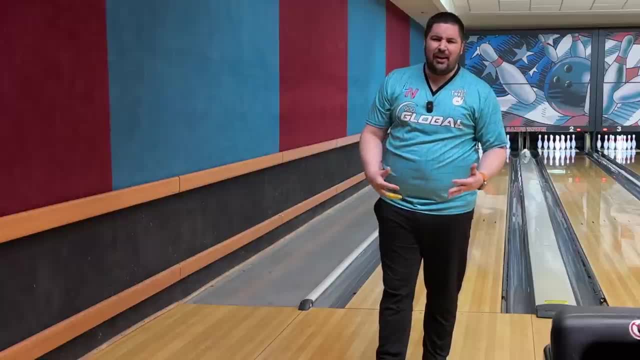 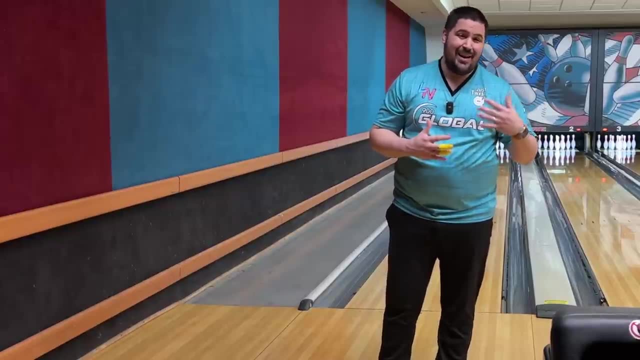 it's not going to over jump, it's not going to hook at my feet, it's going to do all the right things on the fresh, and when i start to kind of look like i'm on a flat 10 territory, that's when i'm going to jump out of the pin down one and get into the pin up one. now, after the shot, i'm going 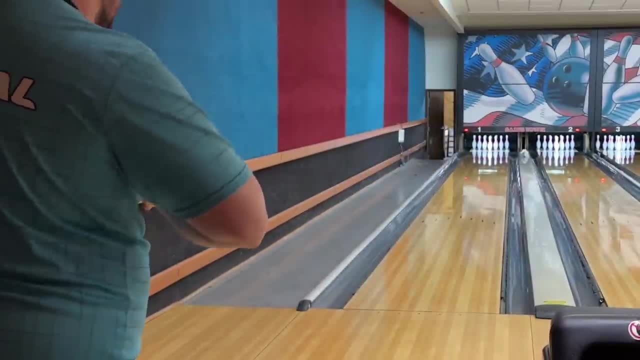 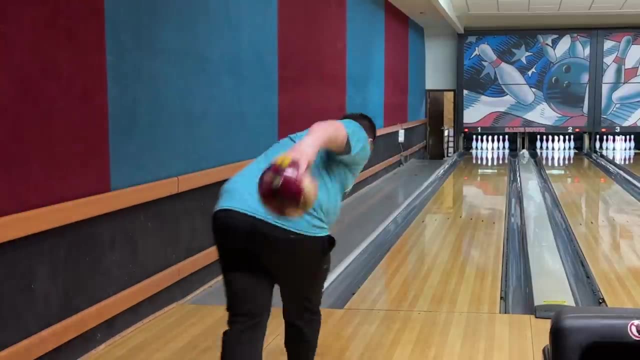 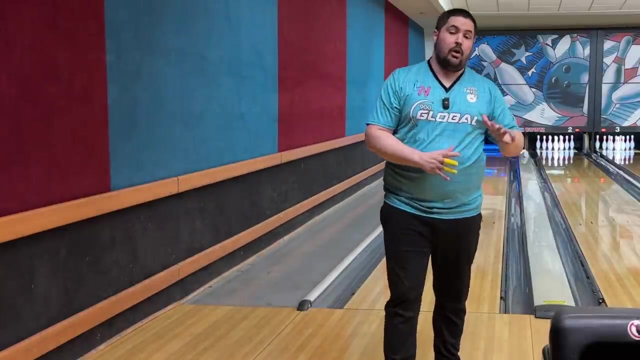 to give you guys a uh, a word of advice, a warning. if you will, we're going to stay in the pin down one repeat, another shot here. there we go. so here's my advice, here's my warning. you, as you guys know, as of a couple years ago now, we can no longer use weight holes. so when you're, 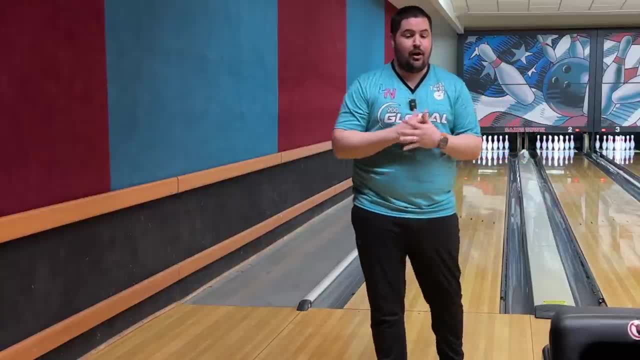 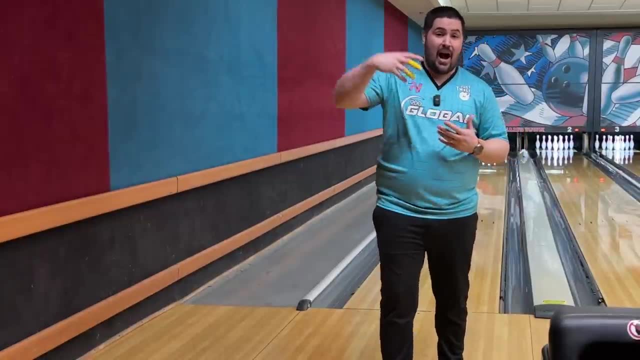 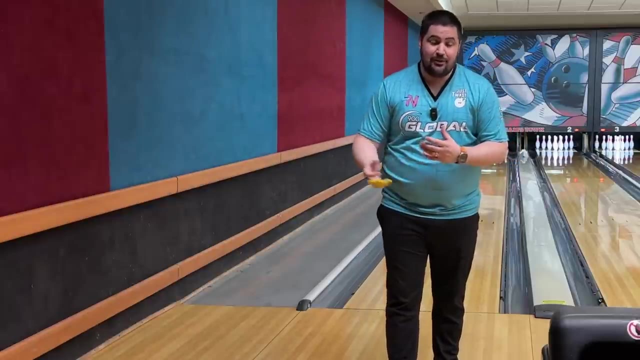 drilling something, pin down, you have to make sure that there's enough differential in the bowling ball pre-drilled. so for me i typically stay with those higher asymmetrical bowling balls with high differentials to start, because if you take a ball that already has a low diff, drill it, pin down and 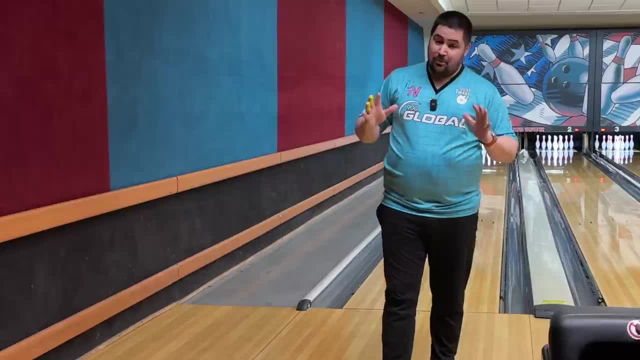 bring that number even lower. it can get pretty ugly. so i'm just letting you know right now: don't take a pin down and bring that number even lower. it can get pretty ugly. so i'm just letting you know right now: don't take like a hustle, drill a pin down and think you're going to get ball motion. 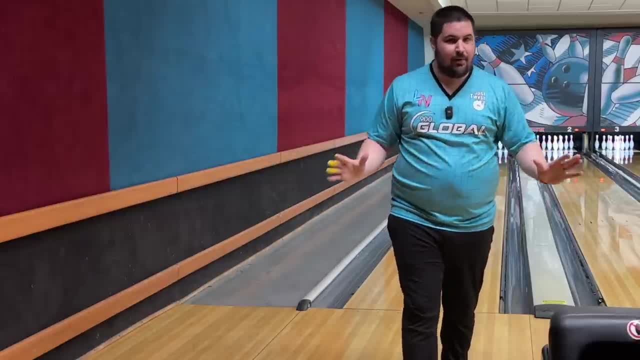 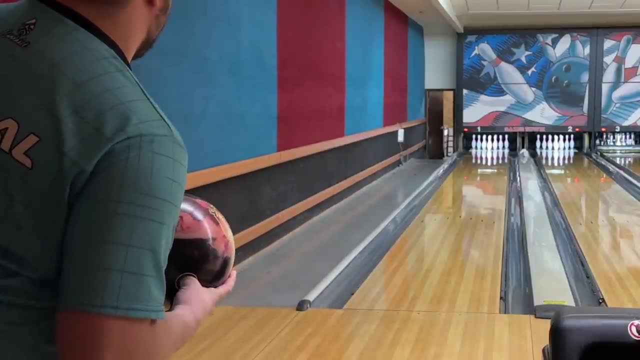 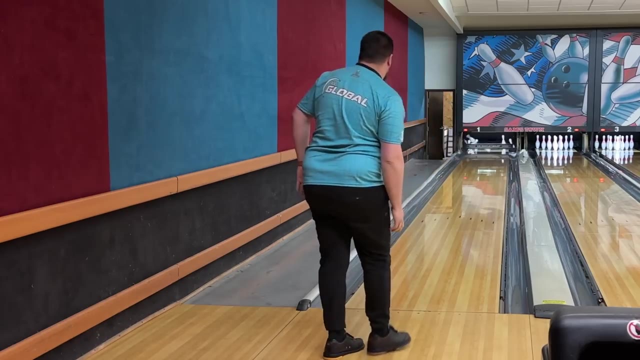 like this: stronger balls pin down. just my advice. all right, that looks too good not to throw at least one more shot, so we'll throw one more with the pin down one and we'll get back into the pin up one. let's go to the pin up one now, all right, so we're going to move back in and get into the.